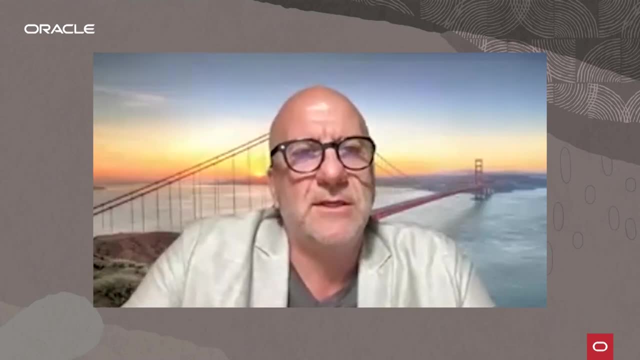 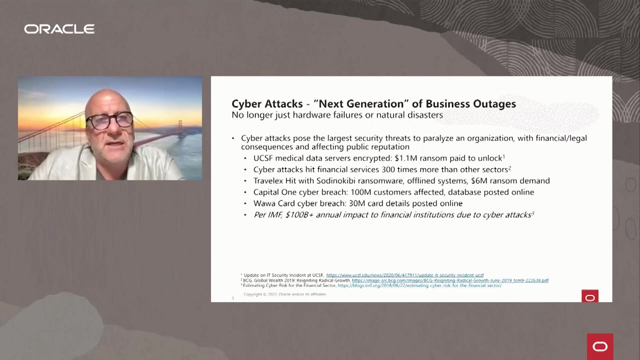 and to focus on is protect and recover. That's what we're going to talk about. Cyber attacks today are really the next generation of business outages. Historically, you know, data protection has always been focused about disaster recovery- Basically what you know we were focusing and 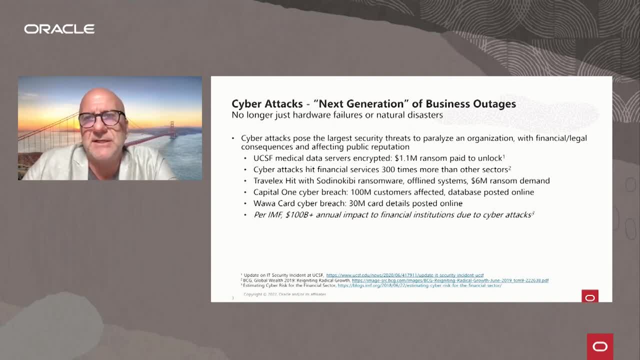 looking at hardware failures, disaster, natural disaster, power failures, those type of things where data loss, of outages, IT issues were kind of a side effect of the problem. Now those cyber attacks are becoming definitely the largest security threats And the point is that 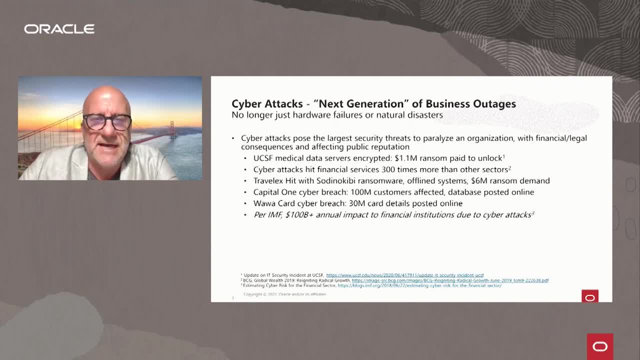 those attacks are really designed specifically to paralyze your IT environment and basically cause business outages that are not only obviously financial legal consequences, but also reputation problems. I have a short list here. There's news every day of ransomware attacks. The first one I have here is, you know, University of California. 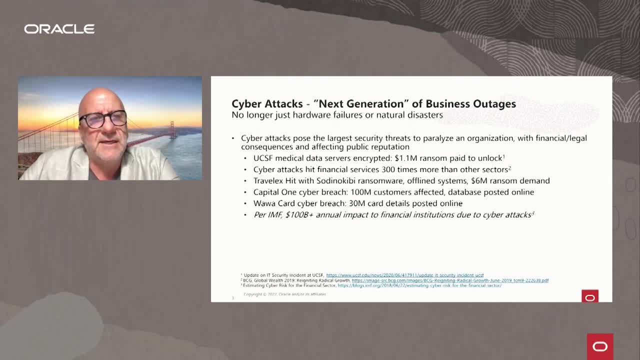 San Francisco. They were attacked where you know, in a cripple locker. you know fashion and all their research data were basically locked and made unavailable to you know, the researchers and everyone, And they didn't have a good backup. They were not. 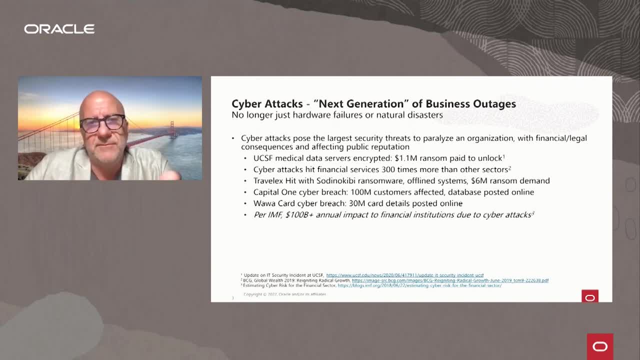 They were not able to recover. They had to pay the ransom, And you know the reason why it made the news is that because it's a public university, so they were forced to publish in their report the fact that they were attacked and also the fact that they had to pay $1.1 million for that to get the data back. 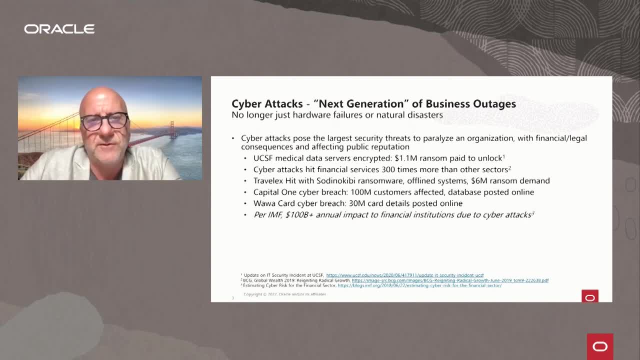 Financial services are attacked, according to a report from Boston Consulting, 300 times more than other sectors, but no one is really in a safe position. All industries, all sectors, all type of companies are constantly attacked. And I have a little more here. 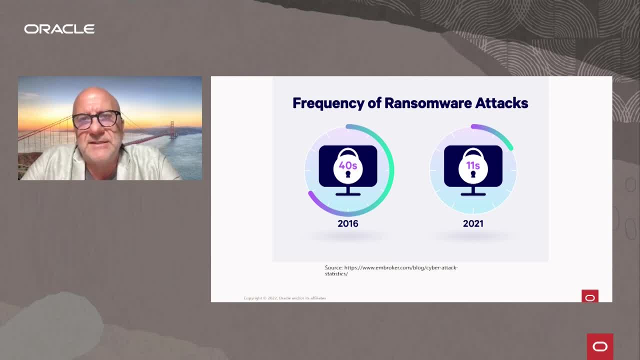 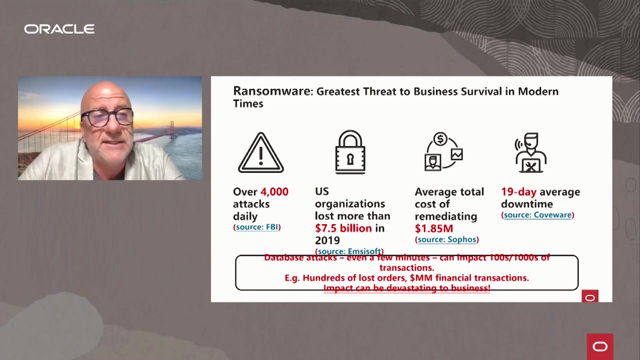 And the frequency of ransomware attacks is growing. We went from, you know, according to this report from InBroker, around one attack every 40 seconds in 2016 to one attack every 11 seconds- And again there are a number of reports, right like the FBI- over 400, 4,000 attacks every day that cost US. organizations more than $7 billion in 2018.. And the average cost to remediate this type of attack is close to $2 million. The probably most staggering statistics about this is the average downtime: 19 days. Now, imagine what it means to be for 19 days without, you know, access to your IT and you know and tools that the company needs to make business, especially you know, given what that's, you know, our main focus. 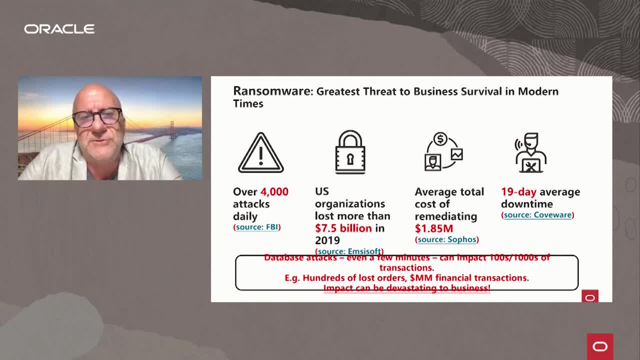 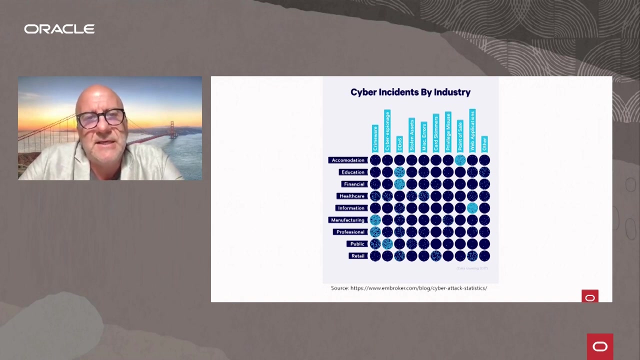 Imagine, if you are for 19 days without access to your databases, what even just a short outage of minutes can impact hundreds of thousands of transactions Right, Which means lost orders. you know means millions of dollars in damages. Imagine being out and not having access to your database for 19 days. 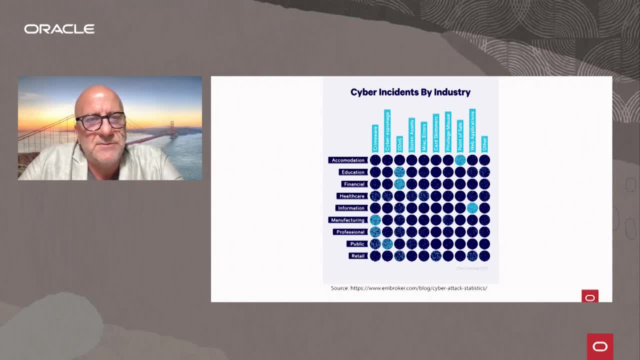 And I was saying, as I was saying before, it's not just a matter of healthcare and financial, which are usually considered the most, you know, targeted industries for ransomware, But really no one is safe And the slides were also from InBroker. 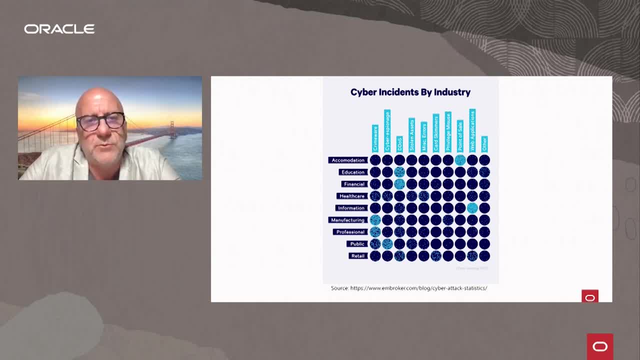 And you have the links here. if you want, You can go and read the reports. It's quite interesting And nobody said that there are different type of attacks and you know different type of attacks can have different effects on different industries. Some are more complicated or more damaging. 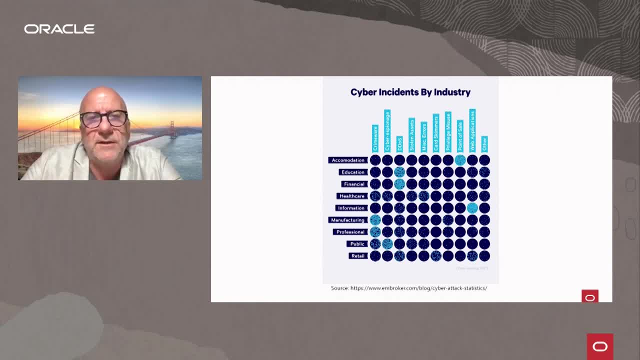 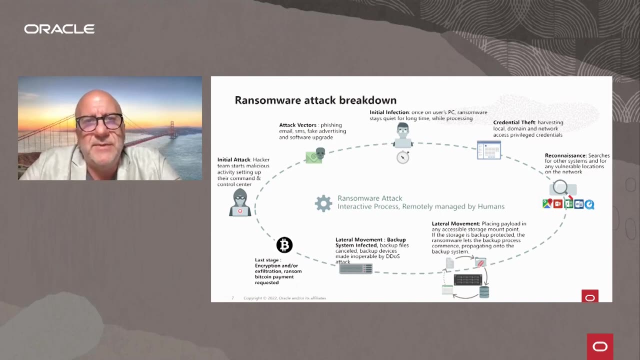 But the point that I want to make here is that, you know, really no one is safe. So what happens? What are we really talking about when we talk about a ransomware attack? So there is, you know, nowadays, a big, big change. 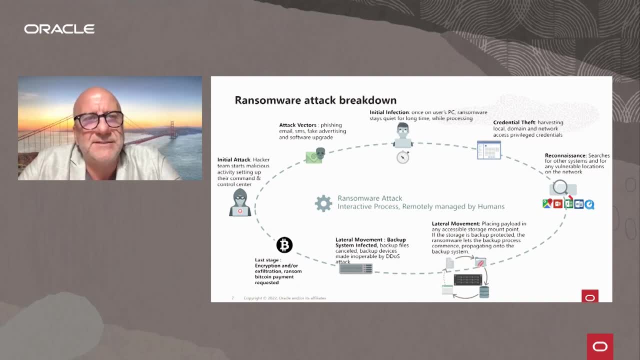 Some also start calling this type of attacks really ransomware as a service. It's not the time anymore where you know it just was one laptop of one employee infected that clicked on an email or something and got just these local files encrypted and maybe a network share or something like that. 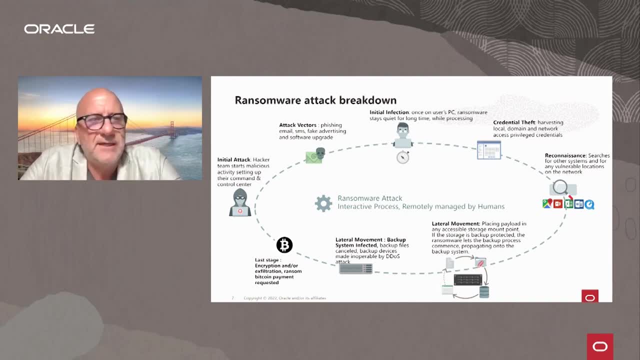 Right. And now attackers are really organized, So they are sophisticated, They are very, very good at what they do And they really set up, you know, some kind of command and control centers. From there they start their operation and they plan for their attacks, targeting and identifying the targets and what they are going to do. 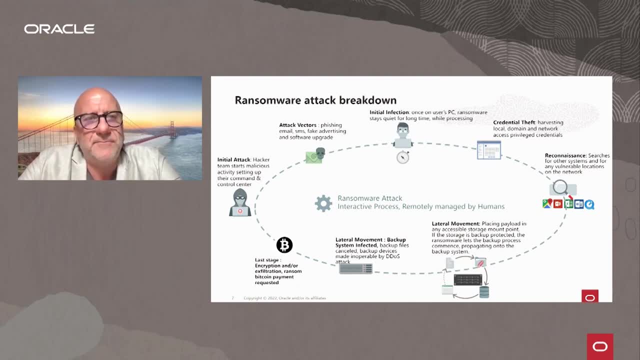 And now then they start pushing out the type of network Right Right, Right Right Right attack vectors that they want to use Again. normally it's just phishing emails. SMS Software upgrades is something that's been seen a few times. 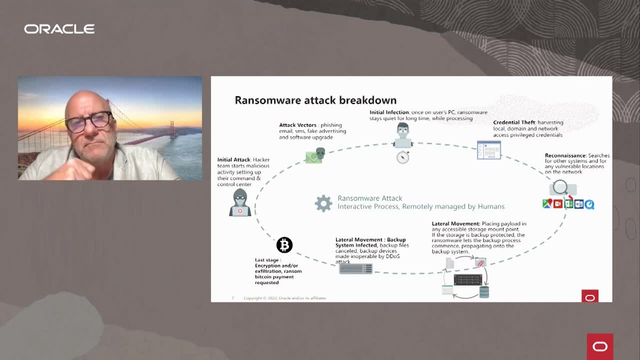 where malware was embedded into a corrupted software upgrade. So customers downloaded an upgrade for a software they owned and sold it, and they were attacked in this way And again. this is not just a simple malware. It's not just the CryptoLocker itself that comes with this. 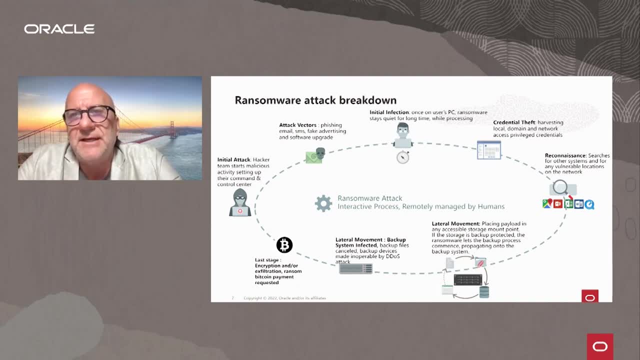 These malwares are really agents that are installed on the target computer And from these command and control centers they really take control of these agents And they can be sitting there for quite some time And from there they start- usually credential harvesting. 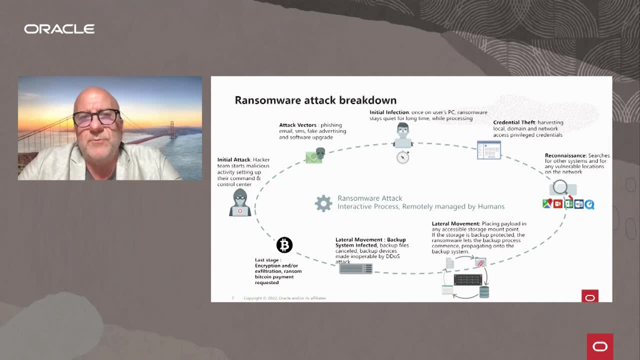 So they start trying to identify what type of users and passwords they can see And you wouldn't believe how many customers- and sometimes I have to say companies that are working and doing outsourcing and doing database management- for example, also for customers- just use Excel files. 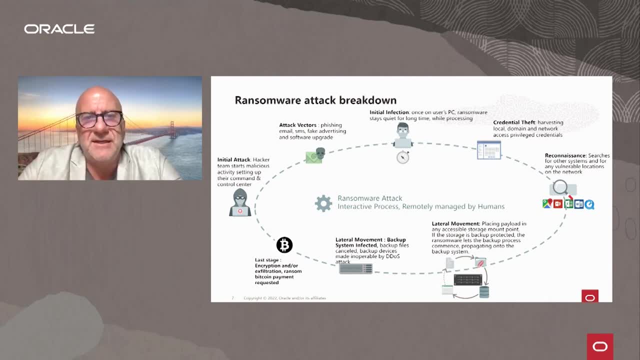 With all the passwords of CIS users and their passwords on Excel files on the desktop of the laptop of the users that are there. So through these agents, once they can get access to that type of information, they start basically identifying what applications are used. 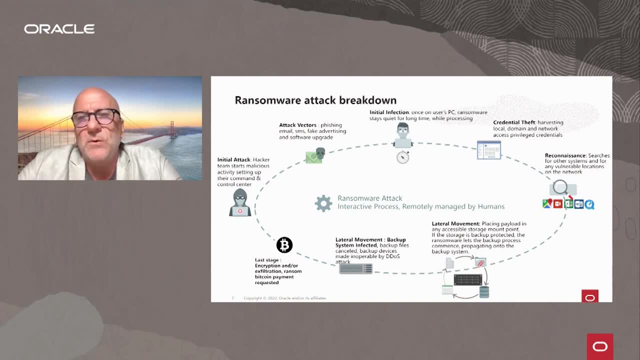 what databases are there, what applications are there, what credentials they can get, And they start moving laterally. They start attacking specifically storage, storage, mount points, again, application databases, whatever they can get onto, with particular attention to backup systems. 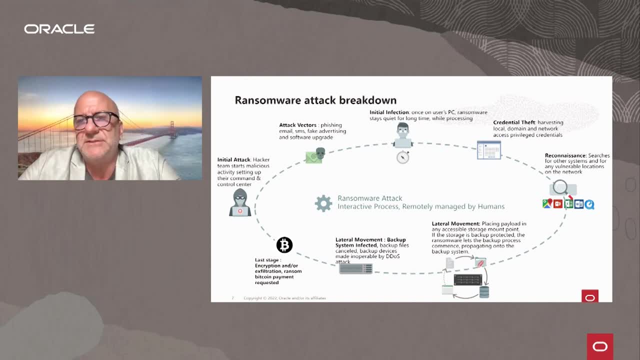 So they try to identify: what type of backup system are you using? They know how to treat them. They know how to random them inoperable, Going to the point of deleting the existing data back ups. rendering backup device or with the objective. of preventing you from recovering, because they know that you know your last resort is OK: restoring from a good backup. If you can't restore from a good backup and you're not losing a lot of data, you can avoid being ransom. 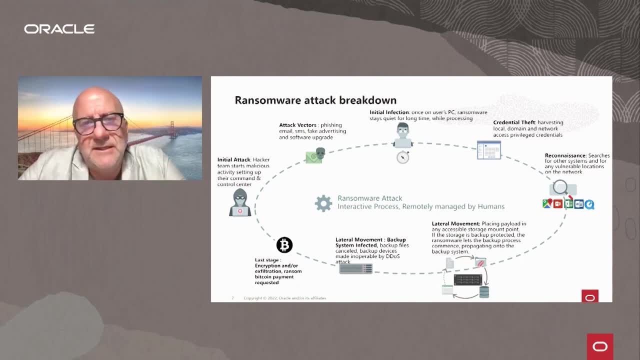 And that's not what they want. So when everything falls, falls in line and everything is done, obviously part of this process, as you are well aware, is also exfiltrating the data. They steal data because they also try to thread on you that. 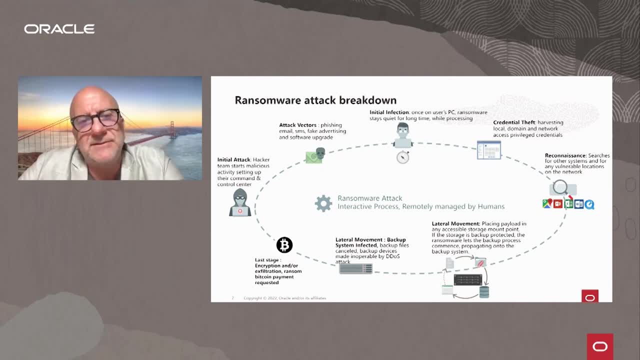 you know, in case you try to ignore our requests and try to restore from backup, But you know that we have a copy of your data and we will publish it. Then you may not be happy. or let me know your business data or your customer data. 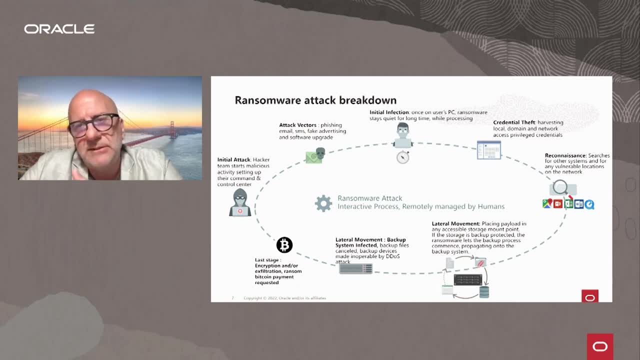 out there on the on the Internet. So they, you know, try to steal data and also, you know, have this second try that they do, And they when, when they're done, they send you a ransom request. And so, again, this is really a sophisticated process. 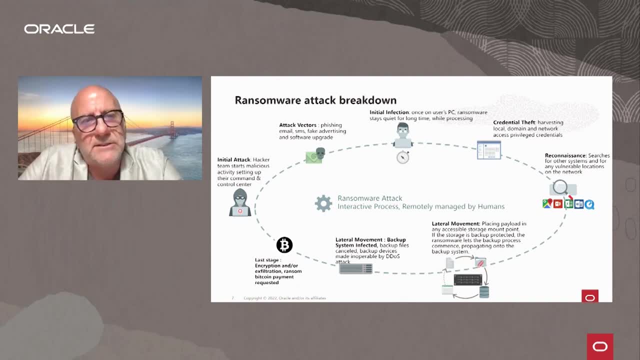 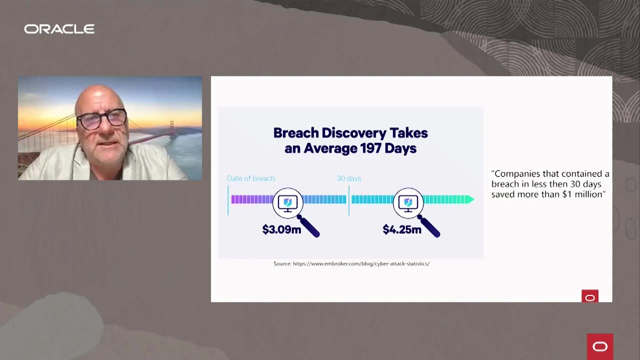 It's not just a simple malware cryptolocker that locks your data, And I was saying that the it takes time to do all of this. The happened right there again, from the same broker report And, on average, the time to discover that the system were breached. 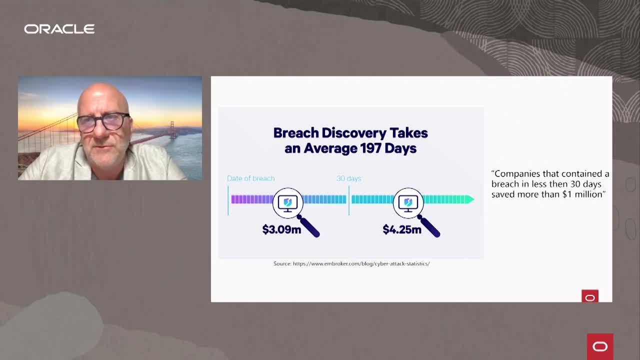 is around 197 days, so almost a year, that that you had some customer, had some agents and and malware and people- criminals- actually lurking and working on the systems, totally unknown. Obviously, the sooner you identify this, the lower is the cost of remediating right. 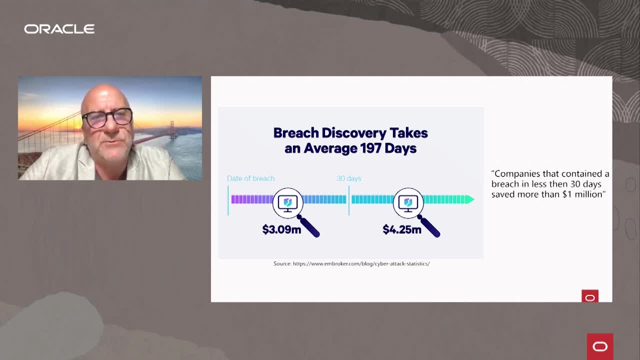 The companies that were able to identify this within 30 days- to identify a breach within 30 days- saved more than 1 million. Again, this is just statistics, but it's really to give you the perspective of how sophisticated this type of attacks are and how long it takes. 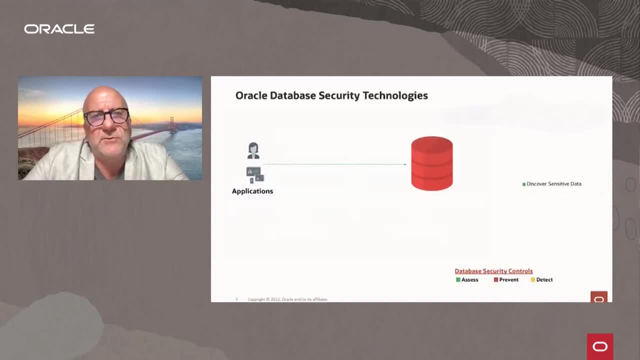 So, focusing on databases specifically, what can you do? And I want to mention this because, again, this is not the case, This is not the focus. But and on on Oracle databases, there's a number of tools, products, so additional products and features and tools that comes with the Oracle database. 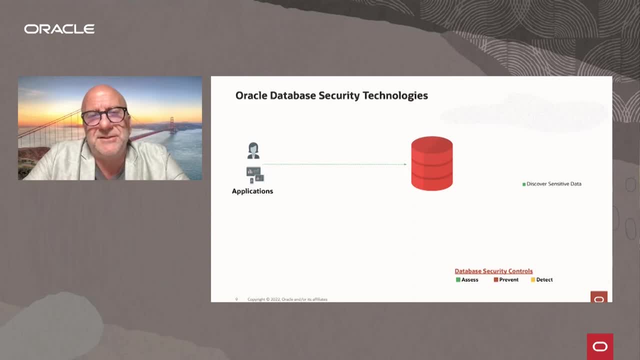 that can help you discovering the breach as early as possible, when it happened, and making the life of those criminals that are trying to do what I just described more complicated. OK, so you have tools like TDE, transparent debt encryption. you can encrypt your data, encrypt the data in your database because, again, 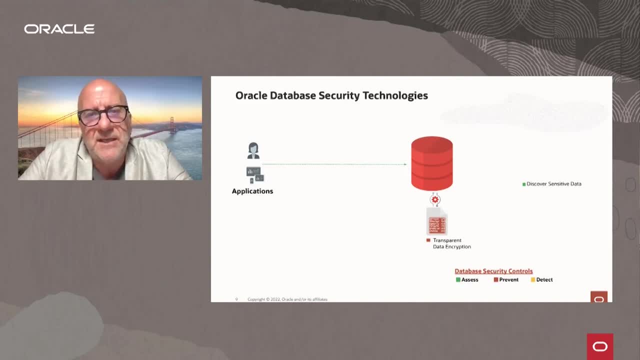 that is the risk of exfiltration. So at this point, even if someone is able to access your database server and steal your database files, they will not be able to to publish the data. They would not be able to find what's in there because the data is encrypted. 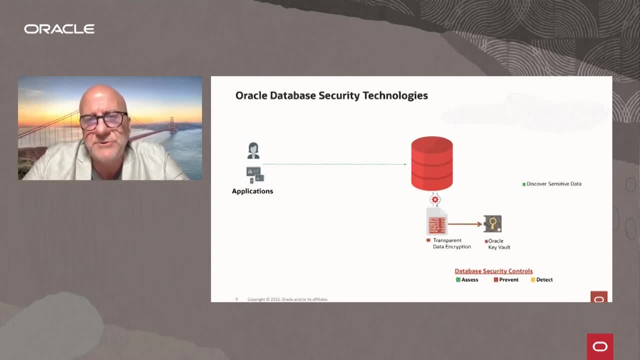 You can use Oracle Key Vault, which is a key manager, to store the TDE encryption keys on an external secure server. So, again, if the database service is attacked, the data are encrypted and the keys are not there. There are other tools, like you know: database vault, data reduction. 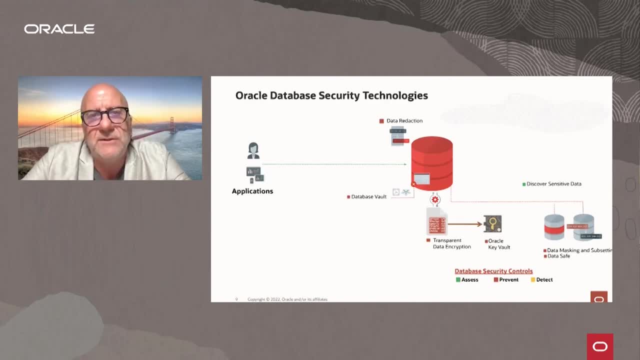 Again, this is not the focus. So I want to really, at this point, give you- and I think Peter later will have something to say about this too, But you know they give you the- the overview of, you know, the all the tools that that are there and the actions that you can take. 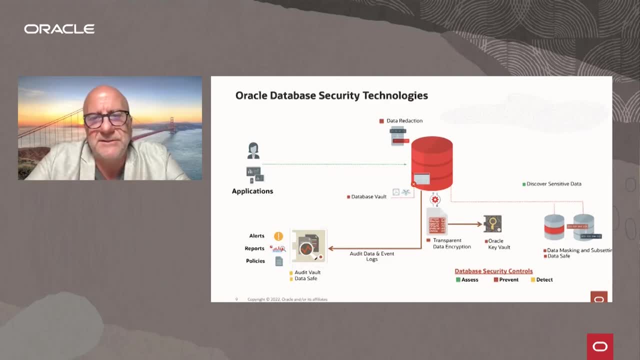 to access, to identify what the situation is, to prevent attacks from happening and also to detect them quickly. Right, So you can use things like database firewall, for example, to filter all the SQL requests going into a database and be able to detect attempts to attack through SQL. 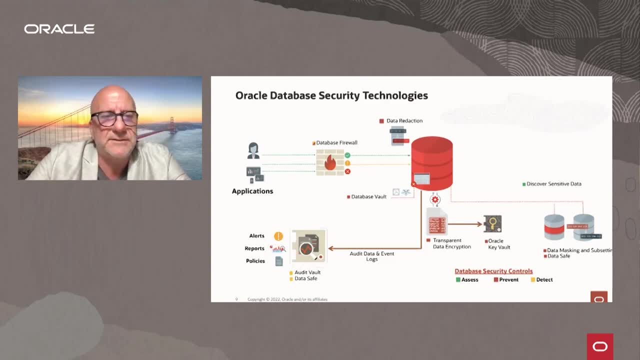 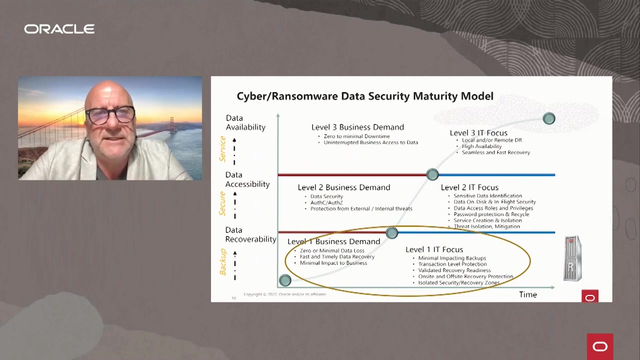 on your database and obviously, detect and report and store everything in data safe and audit vault where you can run reports And again. all of this with the purpose of identifying as quickly as possible that breach happened and to limit the risk of those side effects of stealing data. 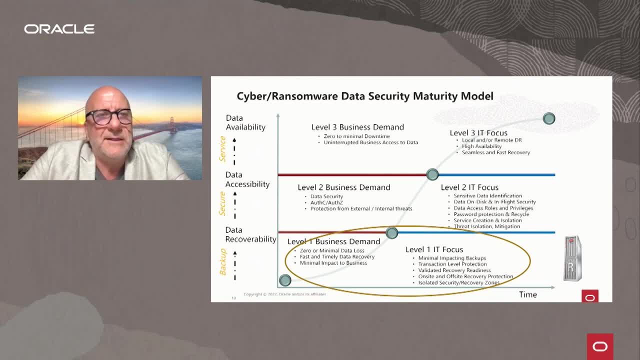 But again, that's not all, And if you don't, you look at this. this is an example of the data security maturity model. the foundation is always data recoverability. The first thing that you should look at is make sure that, whatever happens, you have a valid, secure backup of your data. 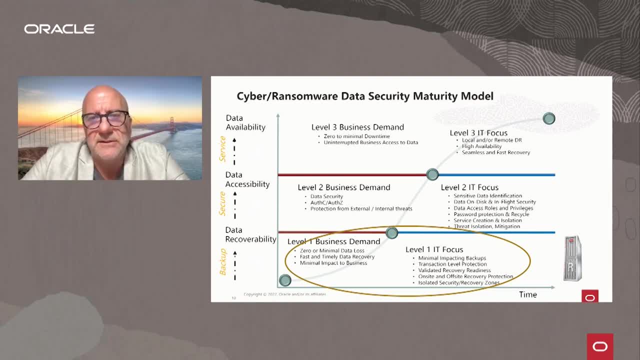 that you can restore quickly and that you can restore up to the closest point in time, right up to the closest time to to the attack. So minimizing data loss, basically zeroing on minimizing data loss, restoring fast, in a timely manner with minimal impact to the business. 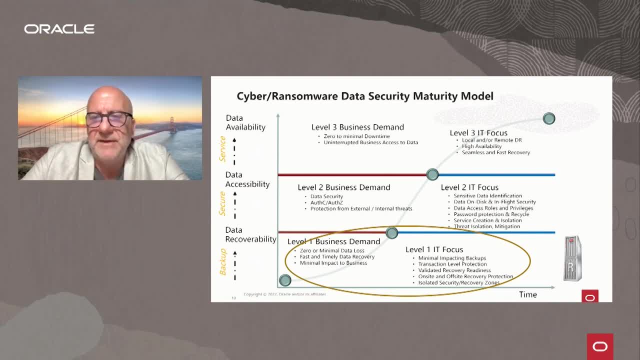 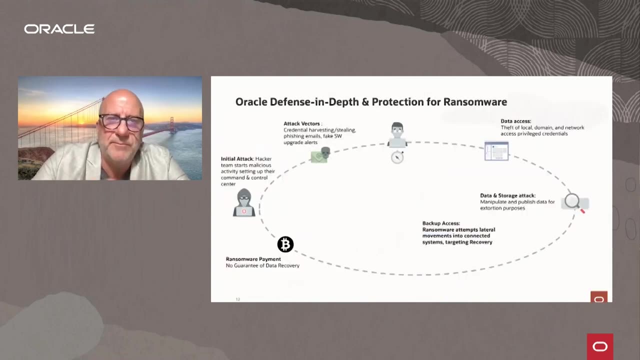 and with validated data, possibly maintaining a copy of your data in an isolated zone where it's even more protected. So that's what I want to focus on And that's what we're going to talk. So, if we put it back on the lifecycle of the Ransomware attack, 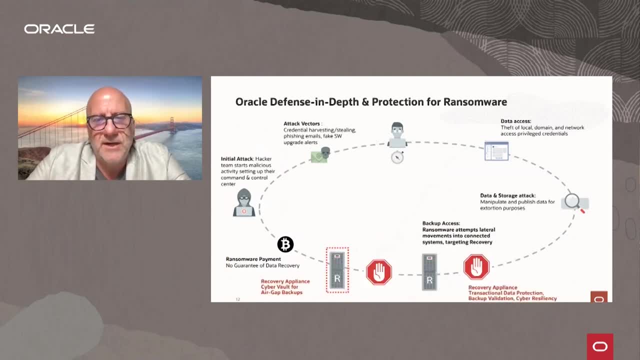 if you want that. I showed you before And this is this is where we are. We are at the point where we want to secure backups. We want the attackers, first of all, not being able to compromise your backups, And we want to be able to have a capture. 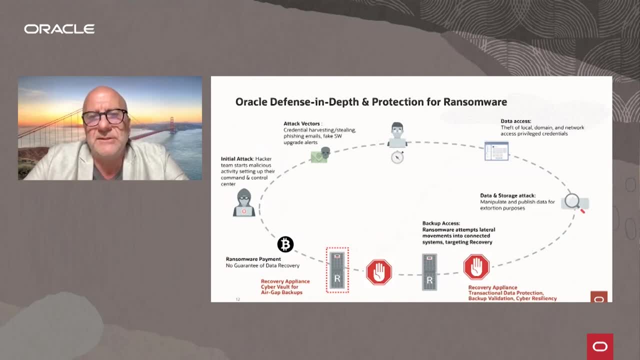 all the data up to the closest point in time to the attack And then going back. there are the other things that I was mentioning, So TD and security on hadn't hadn't exadata infrastructure, So having the database storage not accessible to everyone, for example. 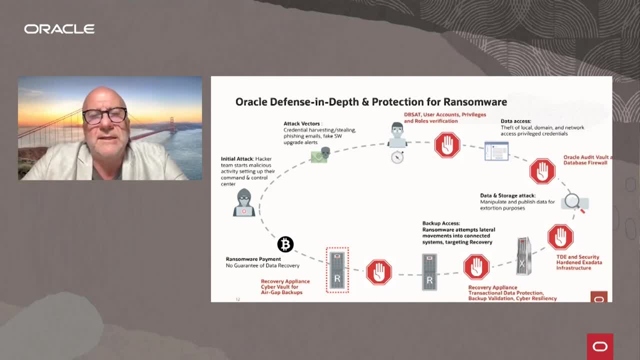 to protect your data using audit vault, firewall or using the security assessment tool to make sure the all the user accounts and privileges and role verification, so all roles are protected, You don't have unsecured users out there, et cetera. So all the things that you can do and that, again, we're not. 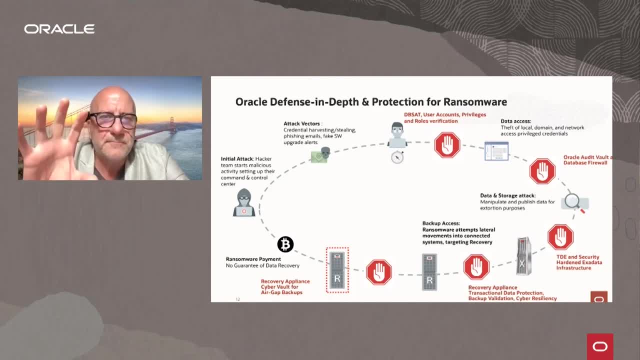 we're not talking more details now, but things that you can do to try to prevent that. But the point is: if it happens, if the attack happens, if it's successful, what can you do? And that's where the zero data. 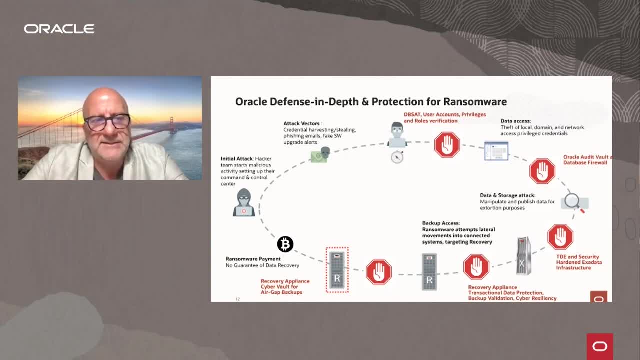 risk recovery appliance comes into place providing exactly those features: the ability to have transaction level protection, the ability to be configured in an air gapped architecture with a secure copy On a normally disconnected location, et cetera, And that's what I would like to talk a little bit more in the next penance. 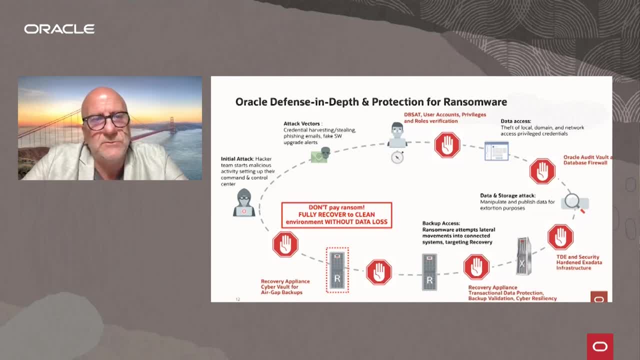 or with the purpose of not paying the ransom, being able to kind of ignore the ransom requests and restore your data and recover and be safe. Also because those are criminals. so there's no guarantee that even if you pay the ransom they will actually give you. 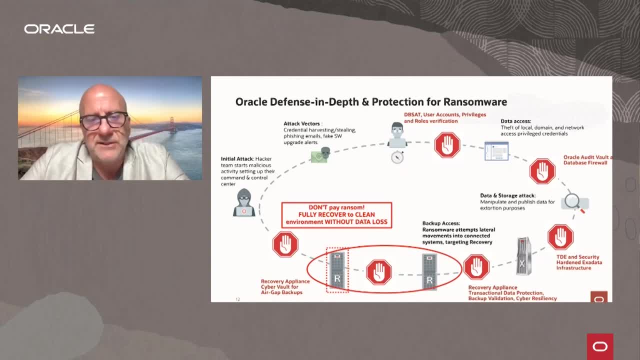 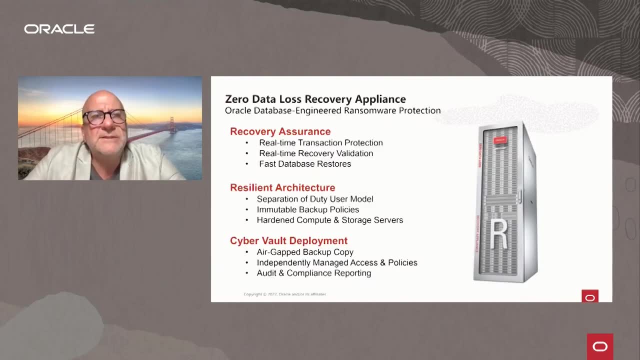 The keys to the crypto data, because they don't care. Well, they care about your money and that's what they want. So let me- let me cover a little bit more details now. which is really the focus again: protect and recover the zero loss recovery appliance and and. 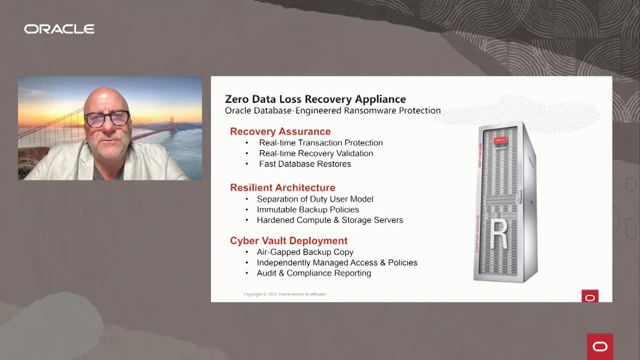 position it and describe how it is. you know good and good solution to help in protecting from ransomware attacks. So we have three pillars. if you want that, you see here recovery issuance ability to have real time transaction protection, real time continuous recovery validation and fast database restore. 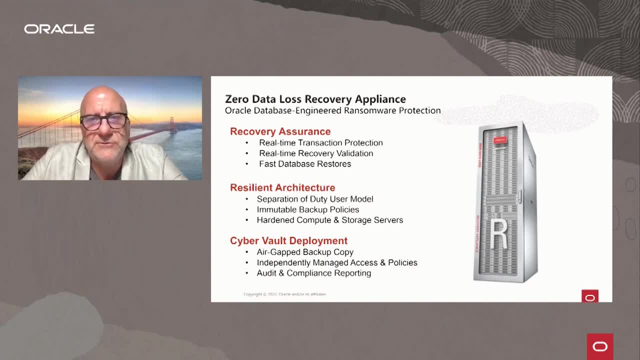 a resilient architectures with separation of duty, user models- And I will talk more details in a moment- Immutable backup policies. You can. you can make sure that no one can alter the backs and you have the same hard and computer storage service I was mentioning before for Exadata, because it's actually built on an Exadata platform. 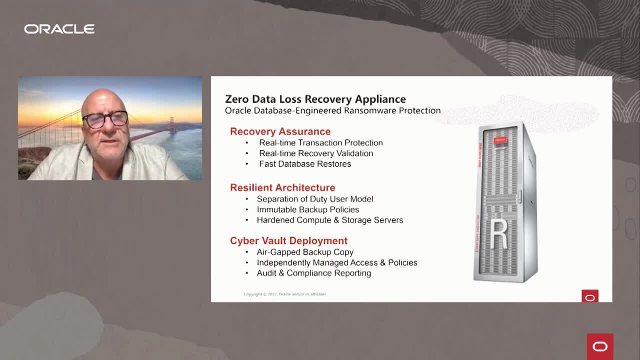 So the hardware is the same as an Exadata server and Exadata system And it means that there is no access to the directly to the storage of the recovery appliances. Backups are not stored in an NFS mount location or something like that, but it's easy for someone to get access to the content of it. 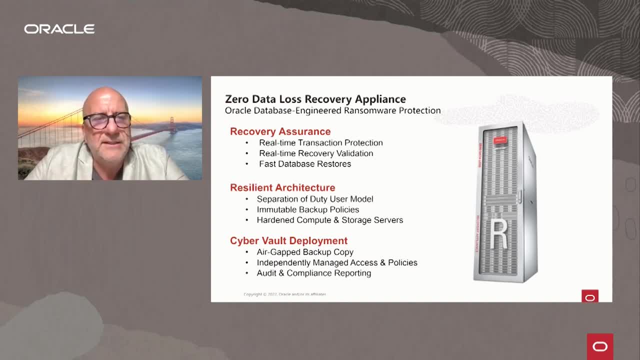 It can only be access to Armin and the cyber vault architect, to the cyber vault deployment, where you can have a narrow gap copy that is normally disconnected from the networks and additional copy of your backups that is actually not accessible regularly on the network. So let's go a little bit into more detail. 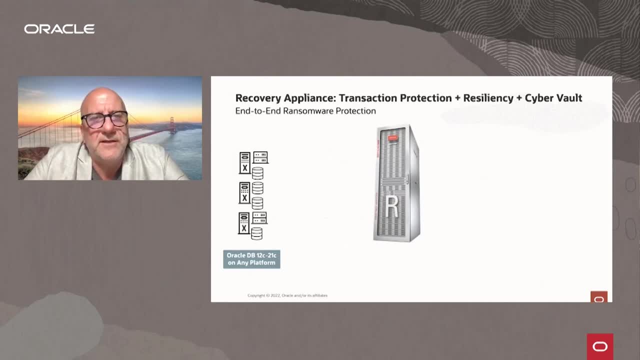 So what it is. for those of you that are Less familiar or never heard about the recovery appliance, Again, it's a. it's a backup appliance and that can be used to backup any Oracle database on any platform, And it provides real time protection. 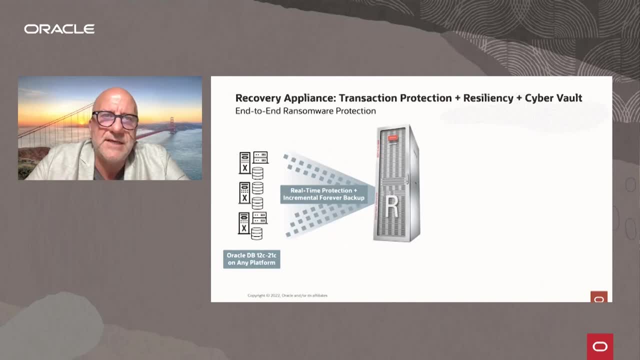 So data are. every block that is updated on an Oracle database is immediately transferred from the database memory to the recovery appliance, And backups are also done in an Incremental, forever fashion. So there's only the changed are are copied, and, and, and they are very fast. 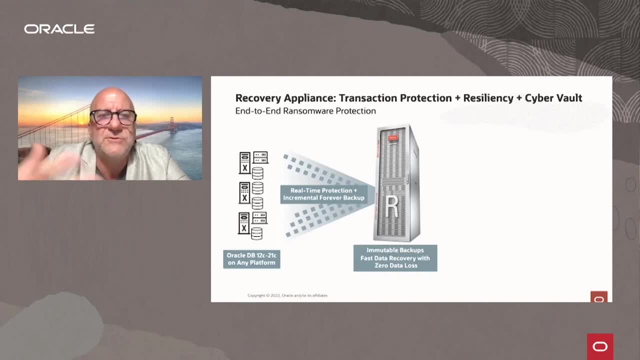 Backups are then virtualized, So they are converted into virtual full backups in the recovery appliance, So when it were a storage store stored as a full backup. it supports immutable backup configuration, so you can configure policies that have a certain retention during which backup cannot be deleted or modified. 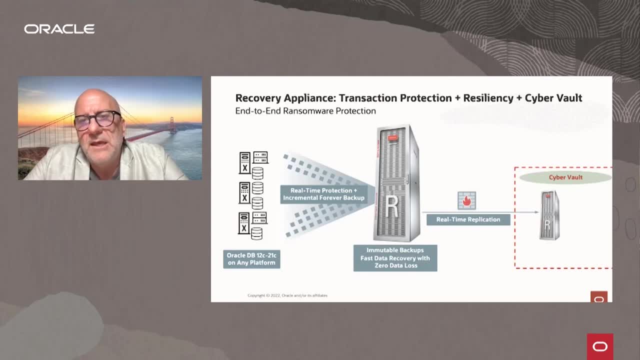 by anyone. As I was saying, it supports a cyber vault architecture, so it can be configured with a replica copy on a location that is normally disconnected. Most of the customers that are doing this are doing this through firewall rules, So they have tools that open the firewall ports. 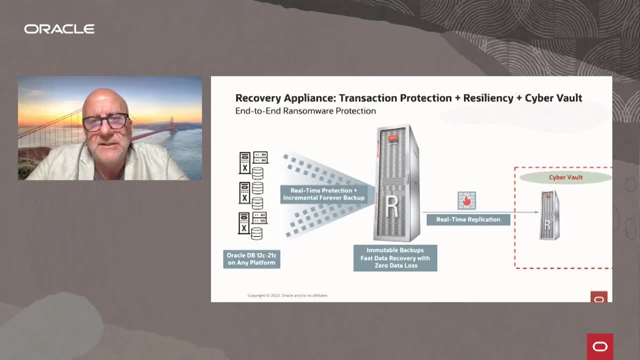 to connect to the cyber vault only at certain intervals. That can be very short, because you only transfer an incremental backup into the cyber vault and then the virtual full is created on the cyber vault as well And and the archive logs. obviously that's what's going to be copied. 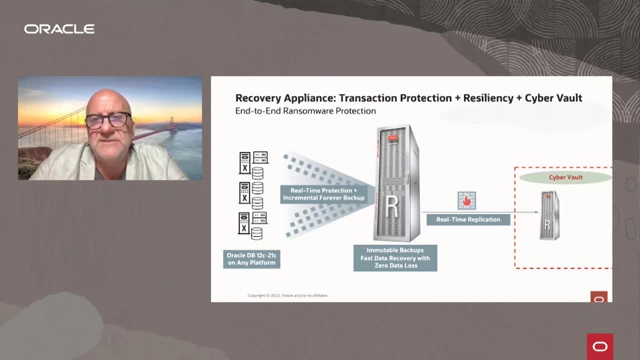 And then the connection is closed and that copy is safe and it's validated locally, So you're sure that it's not tampered with by anyone. Backup can also be copied off site to, for example, to archive storage in an OCI, where you also can define immutable buckets, immutable policies. 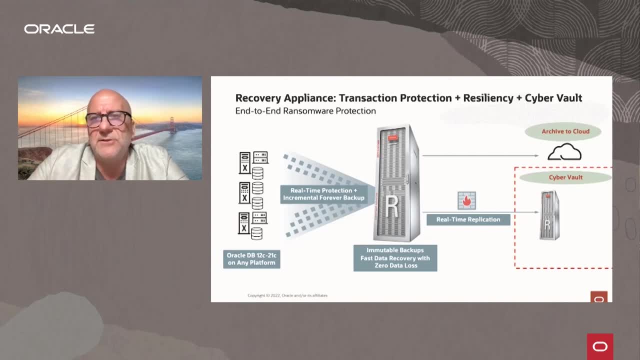 where you can create rules that make the content of the bucket or make the bucket like a warm storage location when you can only write and not delete or update for a certain period of time, And you can also use ZFS storage appliance as an additional target. 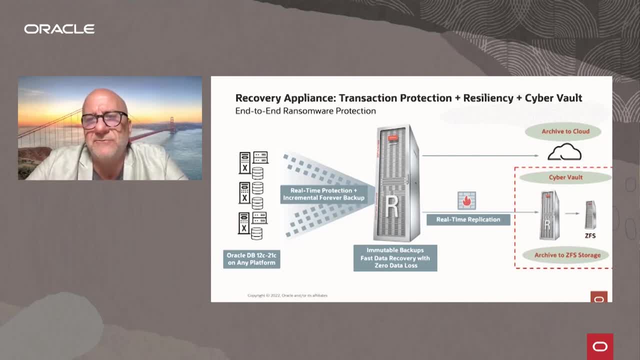 again with the same immutable policies configured, And that can also be the first tab In this example. you see it in the cyber vault, can also be outside of the cyber vault, You can configure it however you like. TDA encryption is supported across the whole lifecycle. 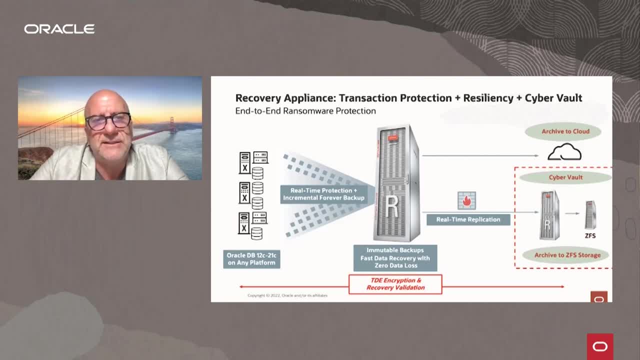 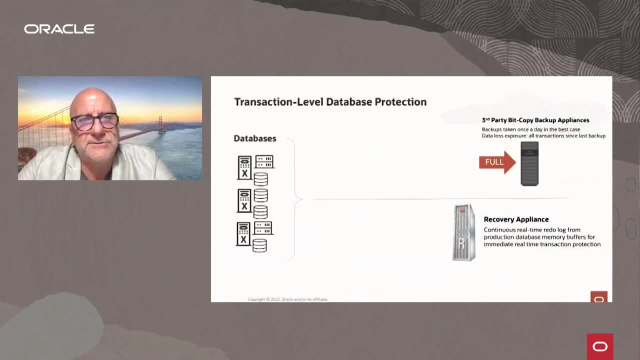 And the important thing is validation of the data. The data is validated at every step. I will get into more details in a moment. So let's talk about transaction level protection, what it means So normally when you back up an Oracle database to a transaction. 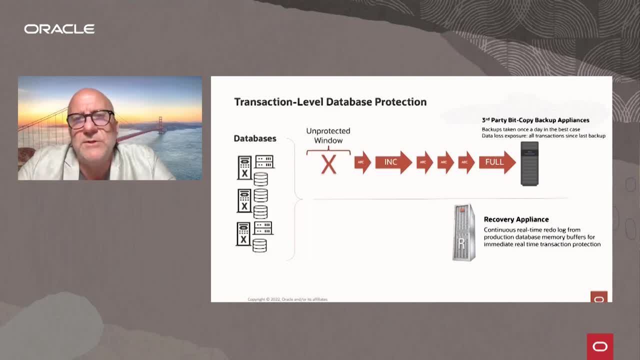 it's a traditional destination. What happens is that you probably want to use a full and incremental backup pattern that is then interlinked with archive log backups, And what happens is that you can recover up to the last backup that you have. So after you back up your last archive log, you start having an unprotected window. 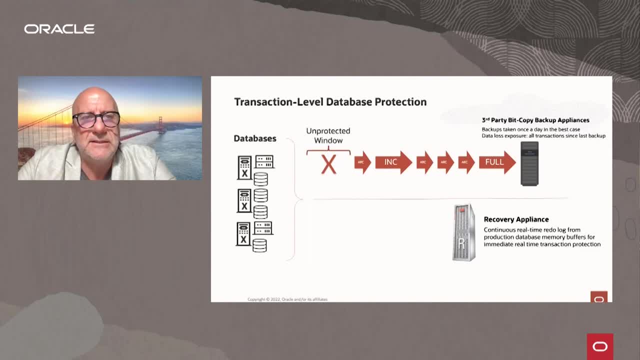 You start having some time where you don't have any protection until the next archive log backup is backed up. So if you have an interval of, let's say, four hours between archive log backups, you potentially lose four hours of your data. So if you have a ransomware attack happening, you may end up losing. If you want to restore from such a type of backup solution, you can lose up to four hours of your work. With recovery appliances, as I was saying, you have a real time protection. Every single block update that happens on an Oracle database is immediately transferred to the recovery appliance. 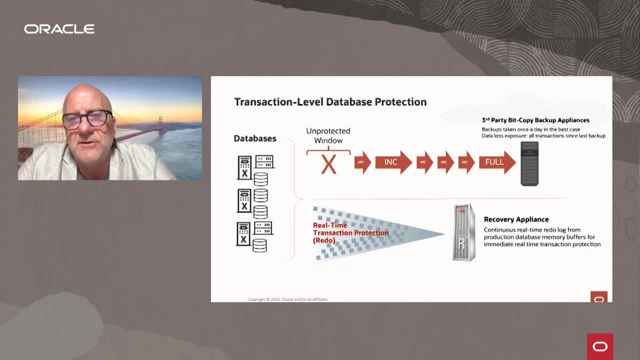 It means that you can recover really up to the last second before a ransomware attack happened. It means that you are not losing any data. You can recover and basically start going from the last transaction before the disaster happened. This is also important When you have multiple. 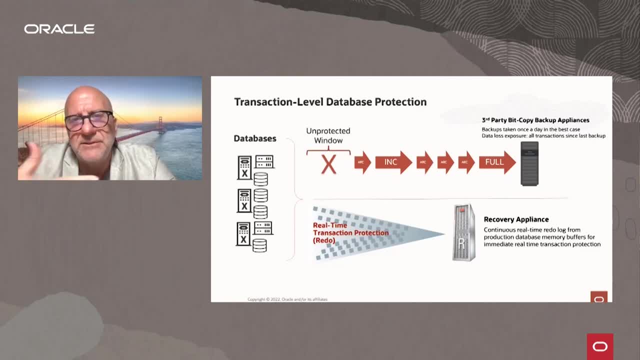 databases. because if you have multiple databases, you want them to be kind of synchronized, right. You want to be able to recover all of them to the same point in time. And if you have different archive log policy backups on different databases, you may end up losing even more time than what you have, just because you know. 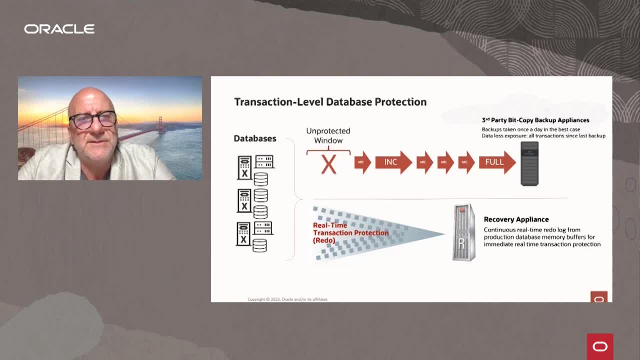 for one of the databases you don't have the same time. They can't recover exactly the same time as another one. So you have to go back a little more With the recovery appliance, as I was saying, you can really go to the last transaction. 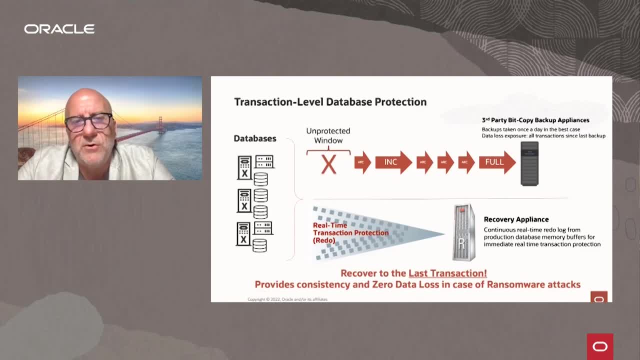 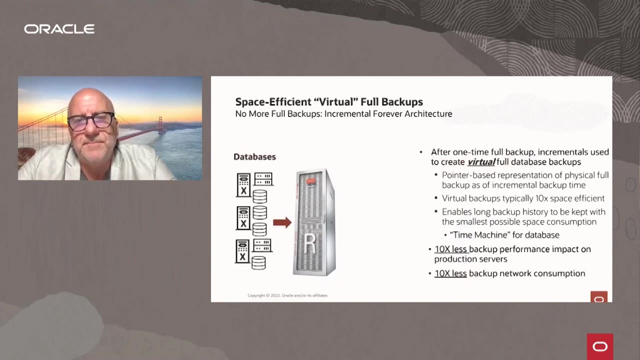 So you have a total consistency that goes above all your database fleet and it can recover really the same. at the same time, The backups, as I was saying, are virtual And what it means is that we use this incremental forever pattern. It means that only the first backup 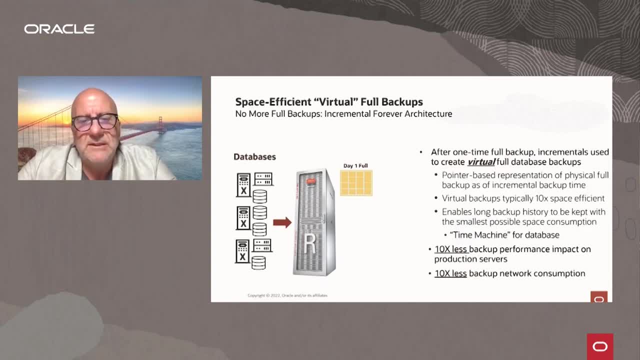 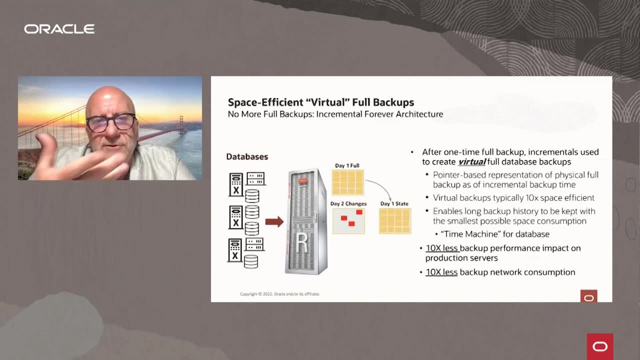 taken to a recovery appliance is a full backup And after that, for the life of the database, you are only taking incremental backups. On day one you have your obviously day one backup, which is the full. On day two, you back up only the changes and only the changed blocks. 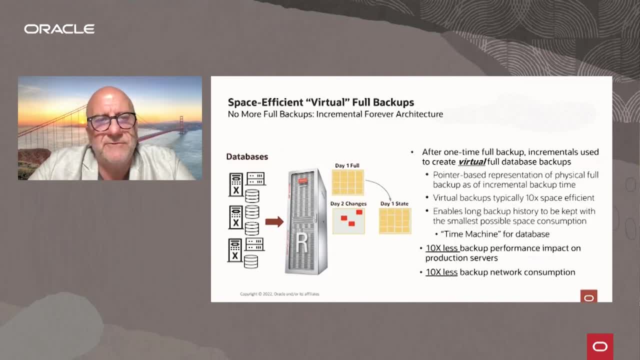 are sent to the recovery appliance. so the backup is short, is very fast And inside the recovery appliance a virtual full is created, combining the blocks from the previous day with the blocks of, so the blocks from the full day one with the blocks that. 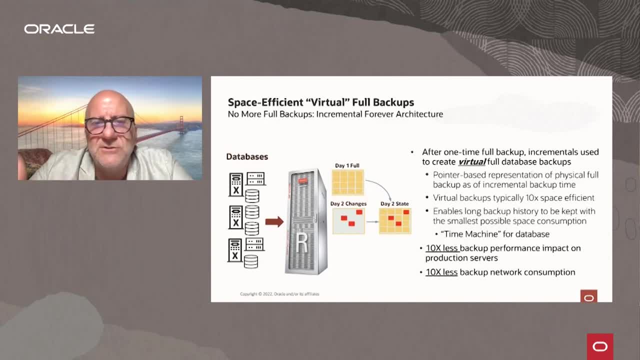 are changed on day two and there's a virtual full is created. There is no merge process, There is no data movement here, It's just this kind of set of virtual pointers creation And you have your full backup representation for day two. 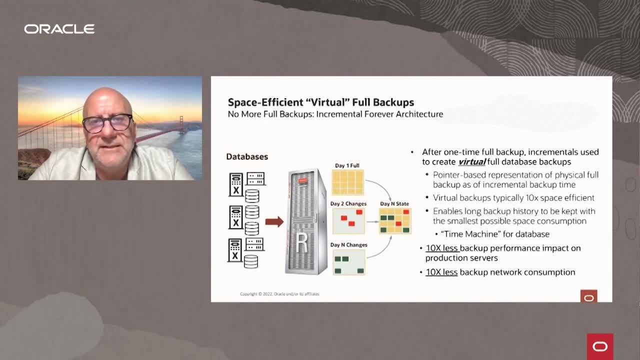 And this keeps going forever. There's no need of taking a full backup anymore, And this allows us To have very fast backups. It also means that, again, when you use a cyber vault replica, you are only transferring the changes, so only the incrementals, to the cyber vault. 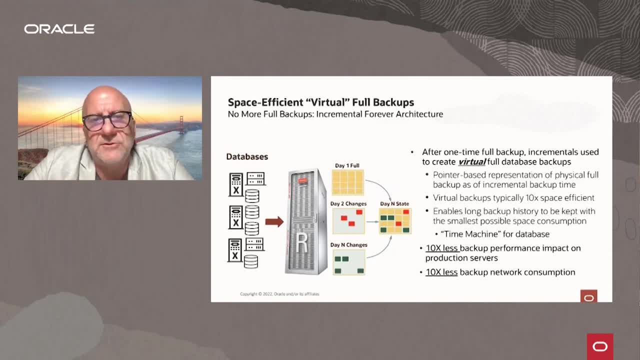 So the cyber vault can be open, always for a very short period of time, where the incremental plus some archive logs are transferred, and then it can be closed. The firewall can be closed again, the virtual full. So this same process Happens also in the cyber vault. The other advantage of this is that when you want to do a restore, you are always restoring a full backup. You don't have to worry about restoring a full and then do the recovery through all the incrementals, Because for every incremental backup you send the recovery plans. 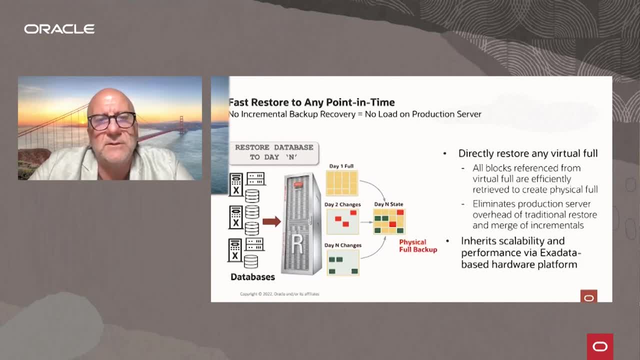 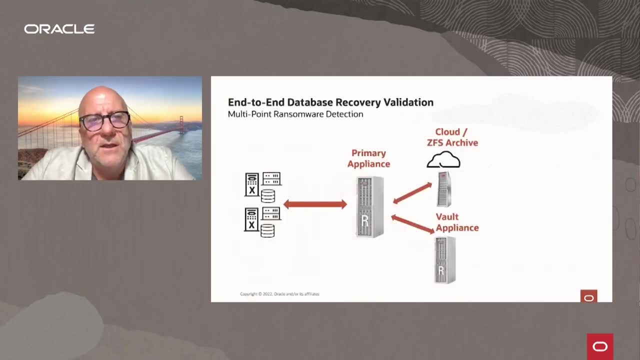 You have a virtual full backup at that time. Okay, so then you can restore to any time that you have protected. The other important topic that we're going to talk about is validation- The recovery plans. Knows what an Oracle block is? 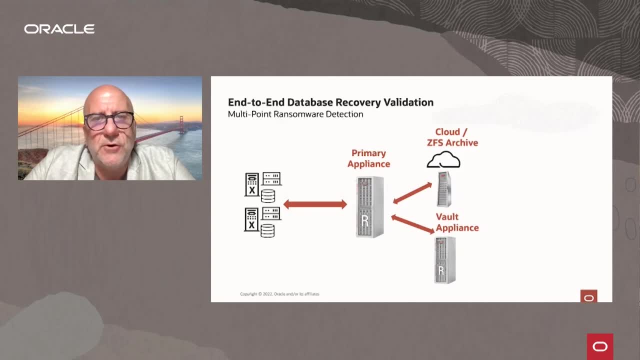 It means that validation is not just based on the simple kind of storage block in an agnostic fashion validation, but it's really done at the Oracle block level And Armin also does the same type of validation. It means that if a ransomware attack, if any type of attack happens on an Oracle database that tries to tamper with Oracle data, 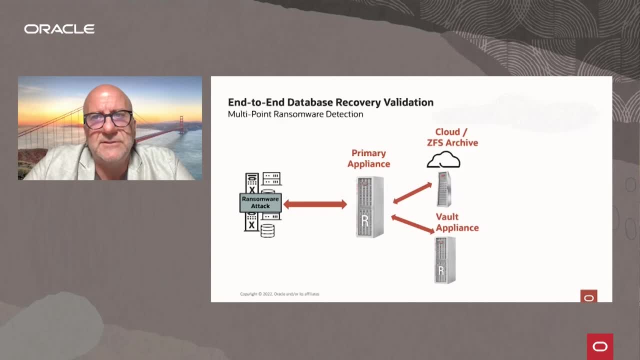 because, again, we just use Armin to transfer the data to the recovery plan. So we only move Oracle blocks and if anything happens and any attempt to tamper with the Oracle data would be detected by Armin because an invalid Oracle block would be detected. 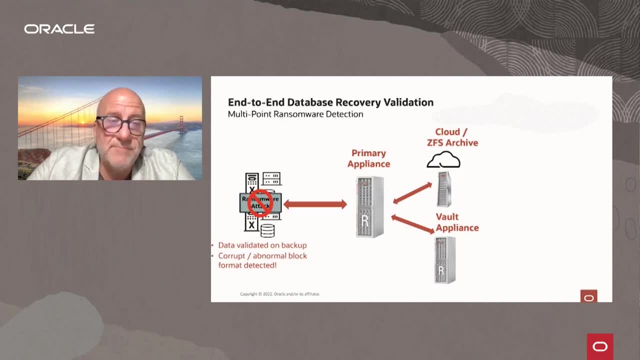 So the backup would be blocked. So if something happens on the database and we want to entertain the idea that someone can try to tamper with an Oracle data on a database server, that data is not going to reach the recovery appliance because Armin would block it. 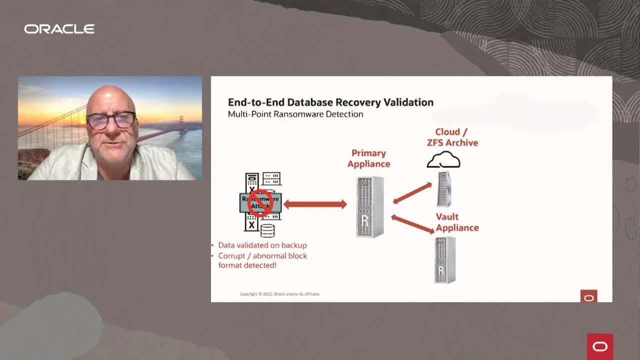 It would be detected the moment Armin tries to create a block. If we assume that we want to consider the idea that something may happen in transit over the network when the data is transferred to the recovery appliance, the same thing happens when the data are received, because when the recovery appliance received the backup data, 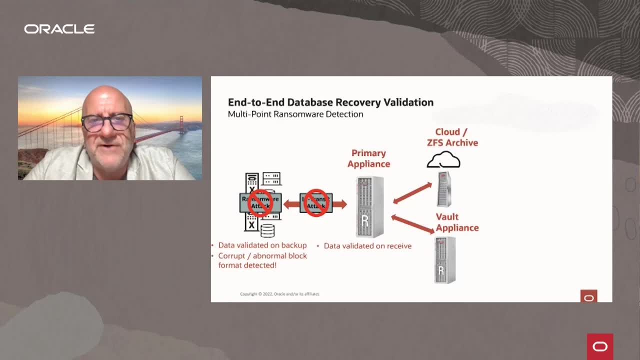 it actually opens the backup file that Armin sent and it indexes all the blocks and validates all the blocks And if an Oracle block has invalid data in it it would be detected. So if we want to assume that anything happens either in transit or on the recovery appliance, 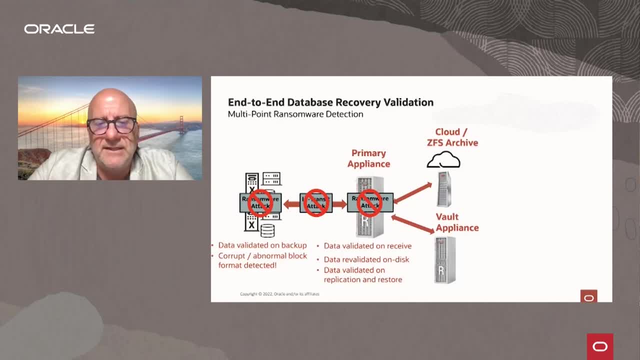 it is detected because it would fail the validation. And the same thing happens at every step. When it's copied to a ZFS destination, to a cloud, again data movement is done the same way and data is validated again Similarly on the Cyber Vault. 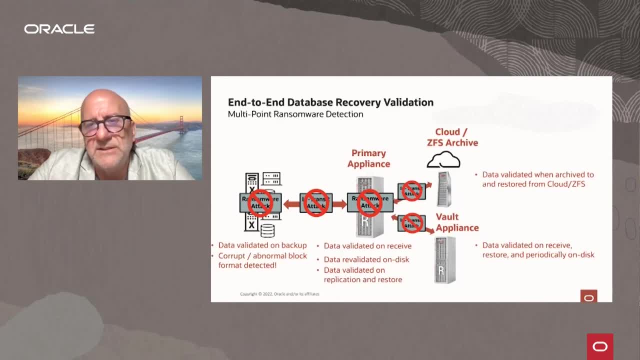 the data is validated when it's transferred and when it's received on the replica appliance in the Cyber Vault. So this also means that we don't need in the Cyber Vault complicated architectures, including database servers, to do validation of the data in the Cyber Vault. 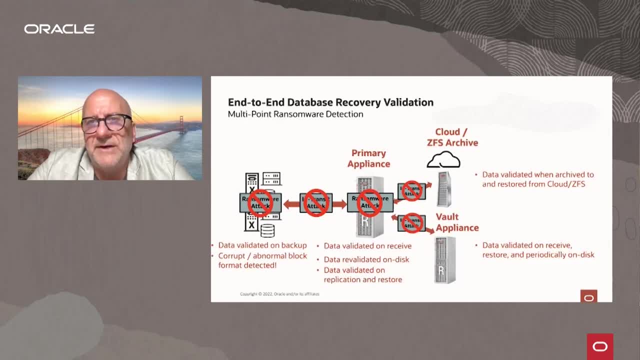 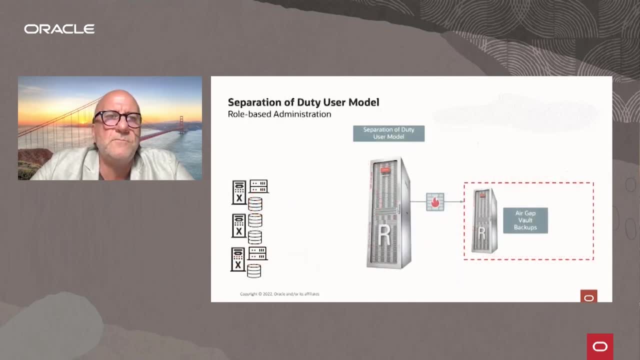 because the validation is done by the recovery appliance itself. So if the data is there, it means that it's valid and it's good In terms of separation of duty. what does it mean? It means that you can have DBAs- database administrators that take care of the databases only. 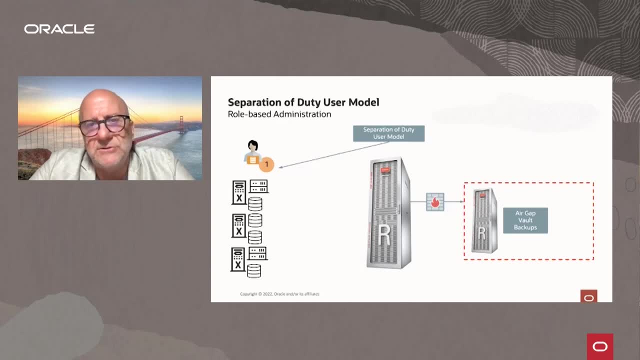 It means that they can initiate backups, They can initiate restores of the databases, but that's it. They have no access to the recovery appliance. and also the recovery appliance can be configured in a way that the DBAs are not allowed to run an ARM and delete backup command to delete specific backups. 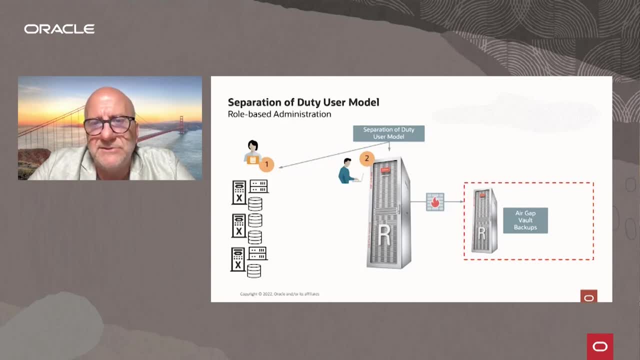 The recovery appliance is managed by recovery appliance administrators. The recovery appliance administrators define the policies on the recovery appliance that determine for how long the backup must be kept. So what is the retention on the recovery appliance? And this is not controlled by the DBAs. it's controlled by the recovery appliance administrators. 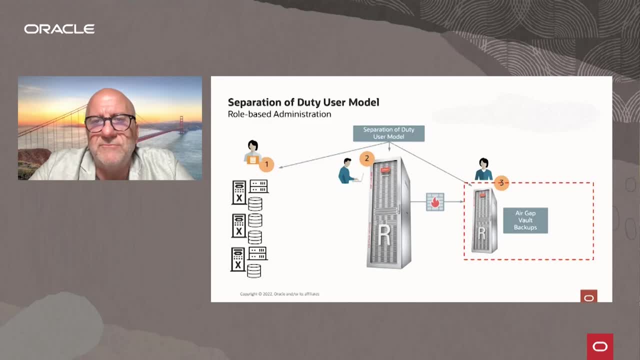 Similarly, recovery appliance administrator in the Cyber Vault. sorry, the recovery appliance in a Cyber Vault can have a different recovery appliance administrators. So different users, different personas, And this limits even more the ability for someone to steal the credentials of DBAs. 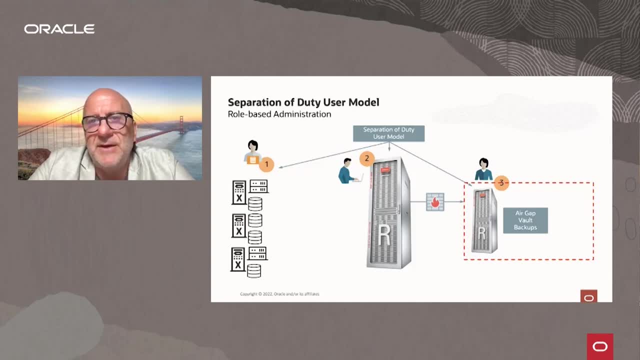 for example, and log into ARM and do a delete backup command and delete all the backups for a certain databases, because it would not work At the same time if someone was able to find the credentials of a recovery appliance administrator may do something on one recovery appliance but not the other one, and also not have access to the databases directly. 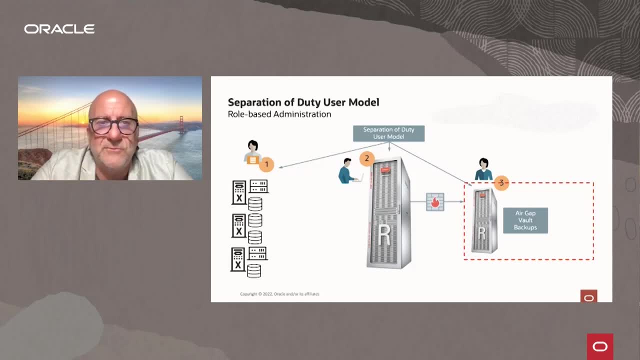 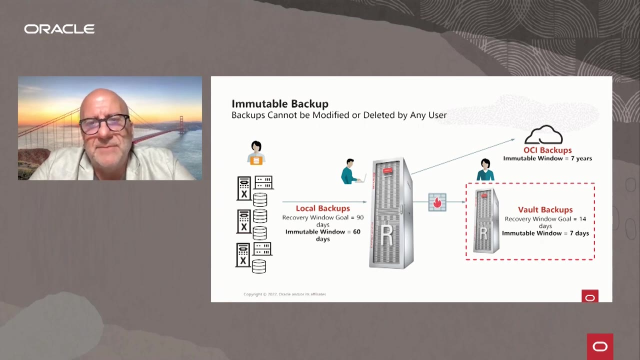 So you know, the process I described before, through which you know there's criminals try to, you know, move laterally across different systems, becomes a lot more complicated. There are also immutable backups that can be configured, So the recovery appliance administrators can set in addition to the recovery window goal. 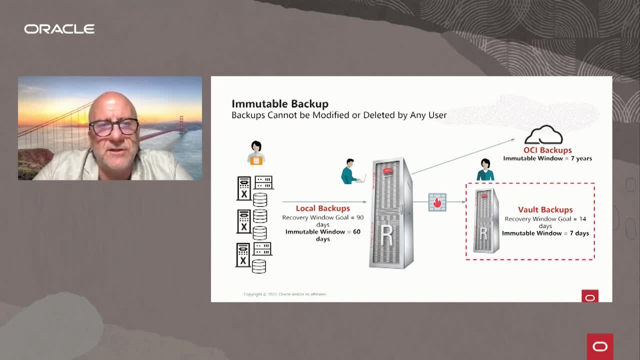 which is the goal, and it's the retention time that is configured for recovery appliance, an immutable window. It means that there is a period of time during which no one can ever change the retention for those backups. An administrator can change the policy and reduce that, but the backup that were taken when the like in this example. 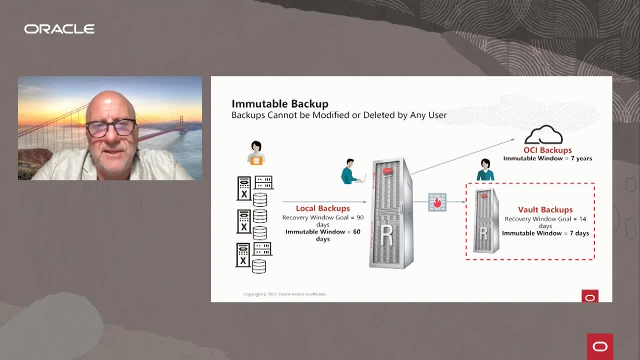 the immutable windows of 60 days will live there for 60 days, no matter what. Similarly, a different policy but with the same concept can be configured in the Cyber Vault and also on OCI buckets, where you can attach what is called retention rules. 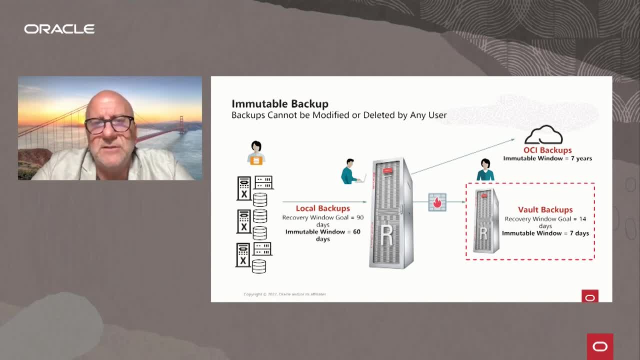 A retention rule on a bucket, making it, as I was saying before, a worm type bucket, and you can set whatever type of retention. It can be seven years, like the example, which is more kind of regulatory compliance type of retention. 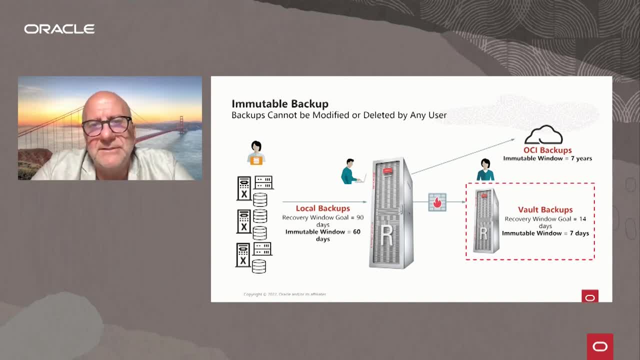 or it can be just, I don't know, seven days or whatever. It's considered usually shorter, just for ransomware protection. So making sure that even if someone can get access to the bucket where the backups are located, it would be impossible to delete them because, yeah, 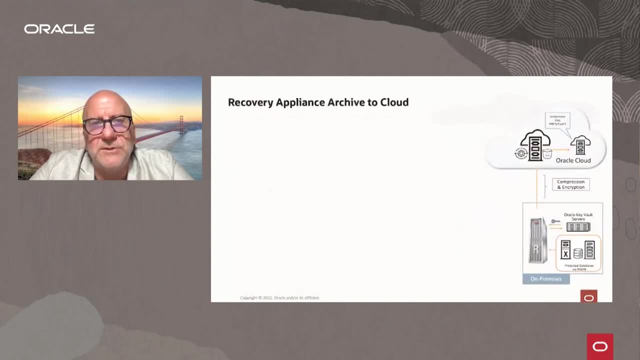 the actual cloud infrastructure would prevent that from happening. When backups are sent to the cloud, as I was saying before, it can be also for compliance reasons not only, but in that case it's more kind of long-term retention type of backup that's sent there. 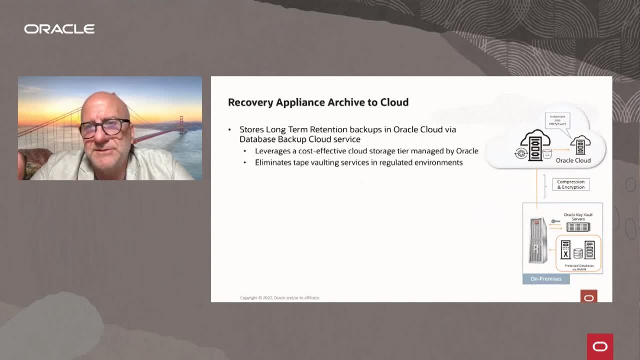 And it can be stored both in standard tier or in the archive tier, which is more cost effective and it eliminates the needs for tape vaulting. So if you have the requirement of storing backups offsite and keeping them for a long period of time, 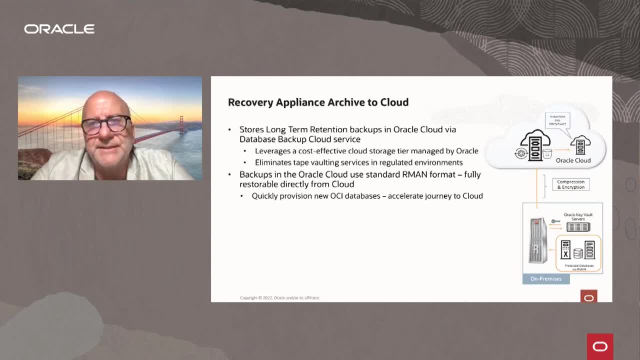 you can do that, sending them from a recovery appliance to the cloud. And those backups sent to the cloud are in standard RMAN format. It means that they can be restored directly without a recovery appliance. So if you assume that you may lose your data center completely and recovery appliance is not available, 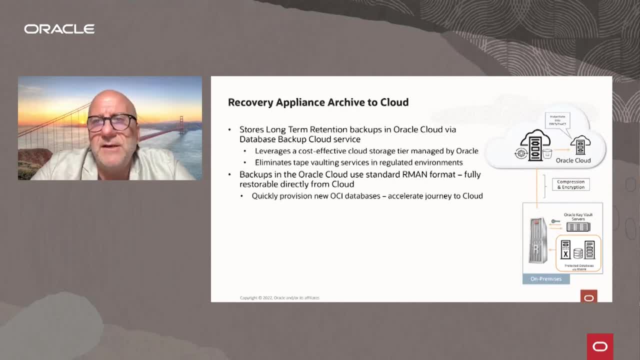 you can still restore, just using RMAN, the backups that are in the cloud buckets And they can also restore into cloud instances directly. So if you do it for compliance and you need to be able to restore for just- I don't know- accessing some old data or whatever for auditing purposes, 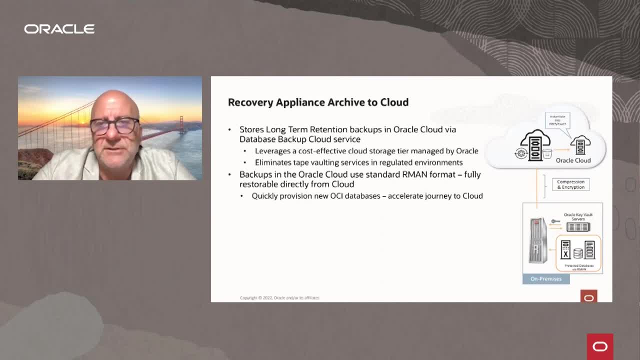 you can spin up an instance in the cloud, restore into a database cloud service or Excel data cloud service, whatever. restore the database there, use it for whatever you need and then you can destroy it and not pay for it anymore. All the backups in the cloud are encrypted. 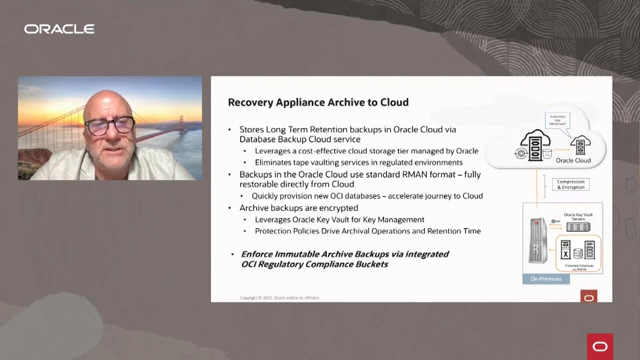 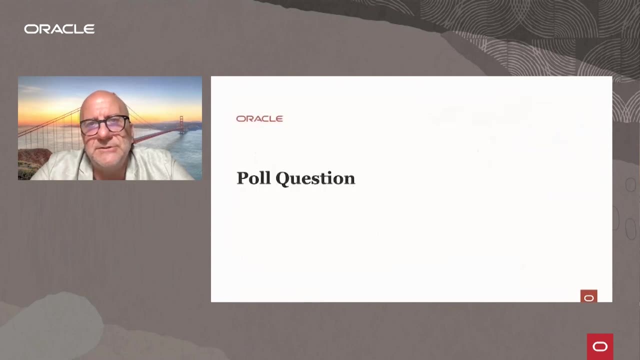 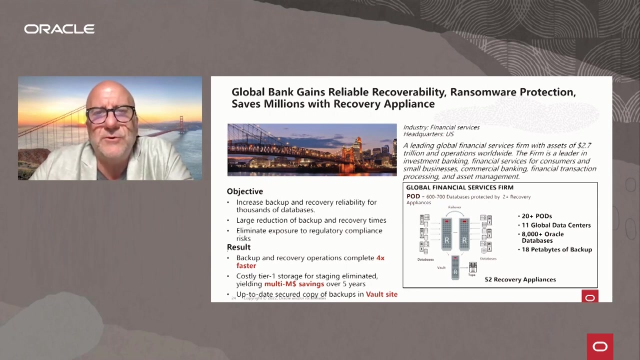 Encryption keys are stored in Oracle Key Vault. And again, buckets. I think this is the third time I'm saying this. already. buckets can be configured as regulatory compliance buckets, So with retention rules preventing deletion. So before closing this, I wanted to mention a few more things. 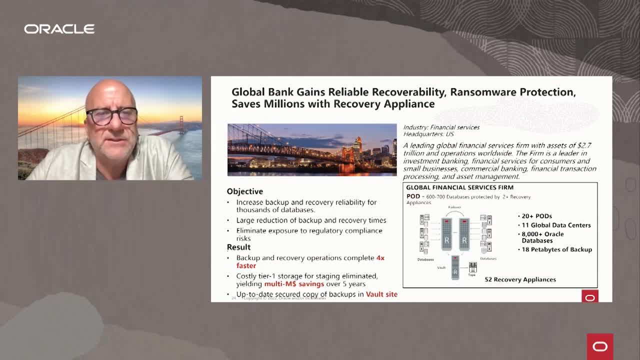 One and a couple of examples of what customers are doing. This is a large global financial institution, Global Bank. They've been using the recovery appliance for some time. They have a quite large environment, A lot of databases- you see 8,000 or more databases- 18 petabytes of backup. 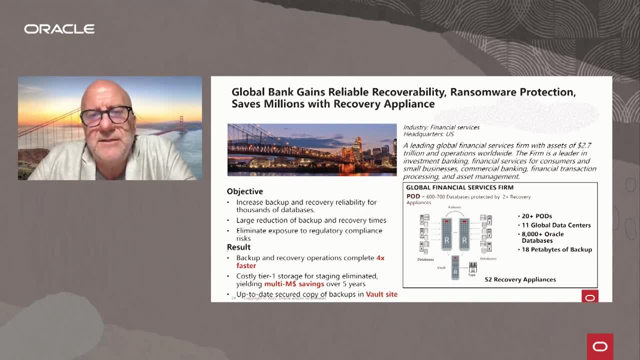 But they recently started using a kind of cyber lockout. So they've been using a kind of cyber vault configuration with a replica recovery appliance And also using traditional tape, so moving data and copying data to tape for an additional layer of protection. They saw their backup and recovery operation improve and being four times faster now. 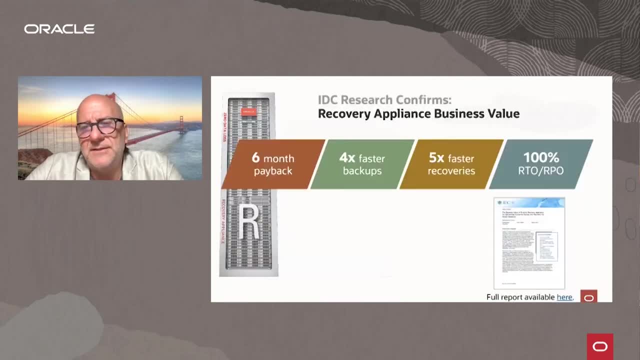 And about savings. that's the other thing that I wanted to mention. I think someone should be able to post the link here, Because when you get the slide you'll be able to find it. That is an interesting report from IDC, specifically on the business value on the recovery appliance. 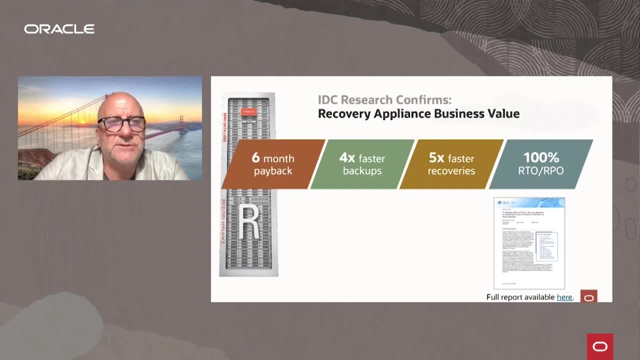 And they did a nice exercise. they interviewed customers, et cetera, And they found out that there's an average six-month payback, four times faster backups, five times faster recoveries and 100% RPO. This is quote one of the customers they interviewed, right? 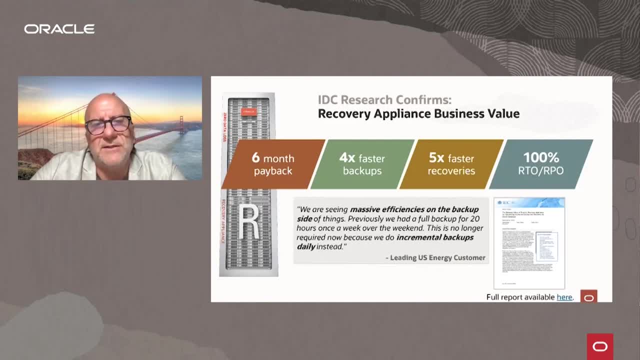 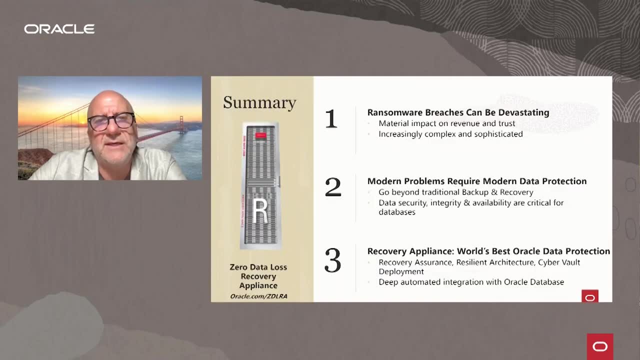 So it's a good improvement of efficiencies. on the backup right, They went to 20 hours once a week And they're now down to a minute in terms of backing up their databases. So, to summarize this, before handing it back to Peter, I hope I didn't take all the time- 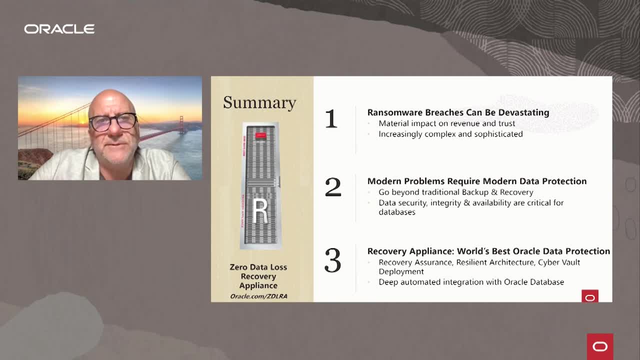 There are some breaches that can be devastating. I think we all agree on this. You know material impact on revenue and also on trust and reputation of the company. Attacks are increasingly complex and sophisticated, and they become more complex and sophisticated by the day. 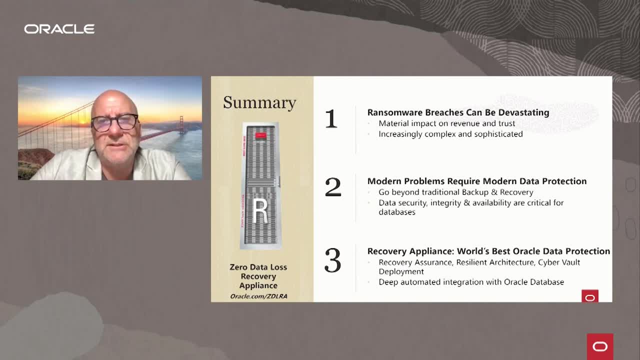 So this type of problems require more than data protection solution, And data protection is, as I was saying before, a pillar and the foundation, if you want, of ransomware protection. You just go beyond traditional backup and recovery And you know you need to include into this also the integrity and availability of your databases. 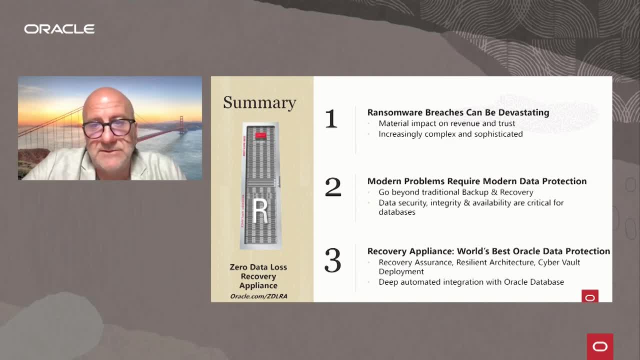 And for these recovery appliances, the world's best Oracle data protection is designed by the same team, Design Armin. So that obviously owns everything around protecting and recovering an Oracle database. It has recovery assurance, It has a resilient architecture. It can be deployed in the cyber world.